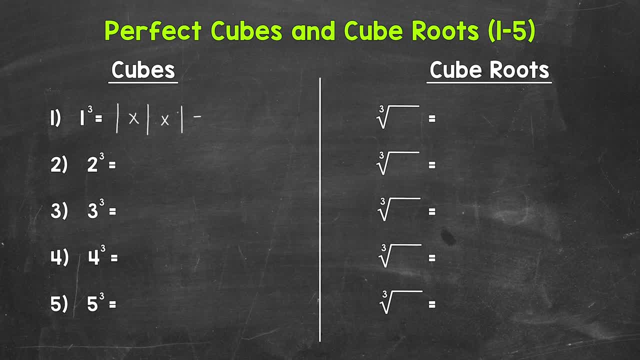 One times one is one times one is one. So one cubed equals one. That means that the cube root of one equals one. Let's move on to number two, where we have two cubed. That means two times two times two. 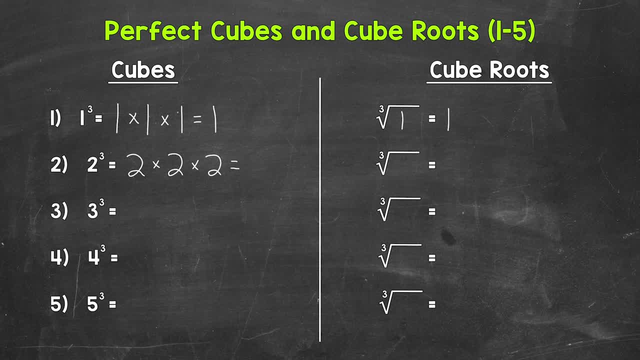 Two times two is four times two is eight. Two cubed equals eight. That means that the cube root of eight Equals two. Let's move on to number three, where we have three cubed. That means three times three times three. 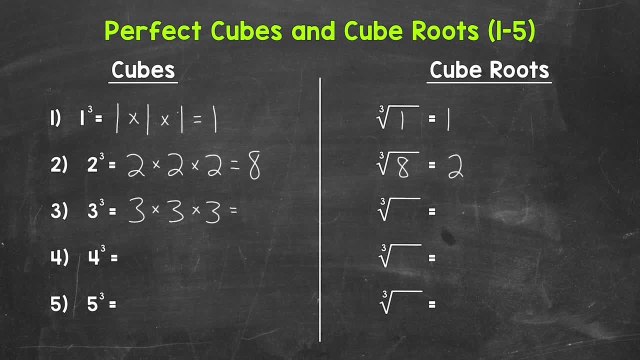 Three times three is nine times three is twenty-seven. Three cubed equals twenty-seven. That means that the cube root of twenty-seven equals three. Let's move on to number four, Where we have four cubed. That means four times four times four. 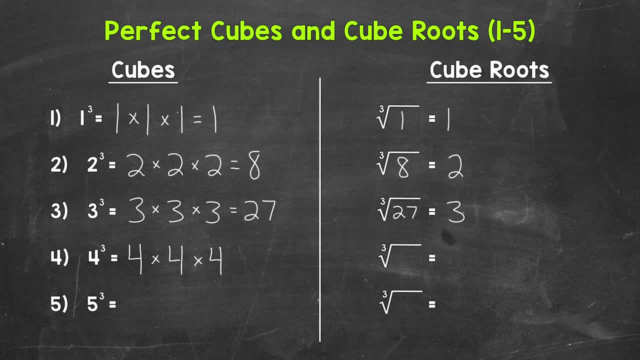 Four times four is sixteen times four is sixty-four. Four cubed equals sixty-four. That means that the cube root of sixty-four equals four. Let's move on to number five, where we have five cubed. That means four cubed. 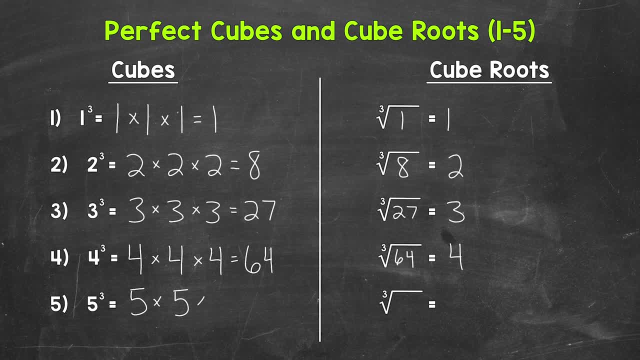 That means five times five times five. Five times five is twenty-five Times five is one hundred twenty-five. Five cubed equals one hundred twenty-five. That means that the cube root of one hundred twenty-five equals five. There you have it. 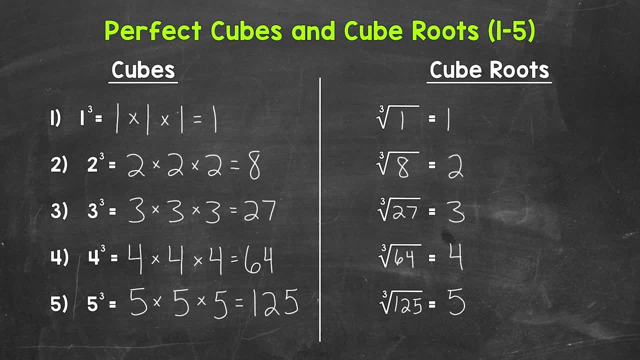 There are the first five perfect cubes and cube roots. Now I would recommend getting down and knowing these five. Once you know these five, work to get down six through ten. This is really going to help with any cubes, cube roots or problems involving cubes and cube roots moving forward. 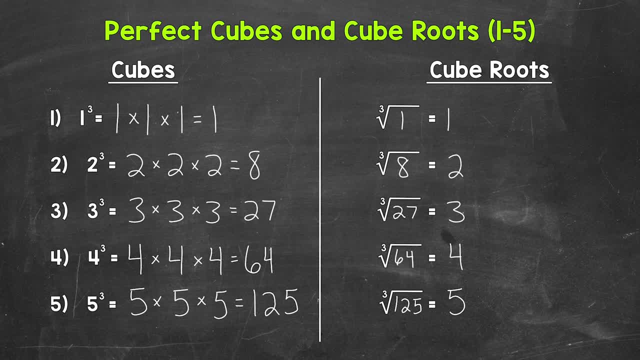 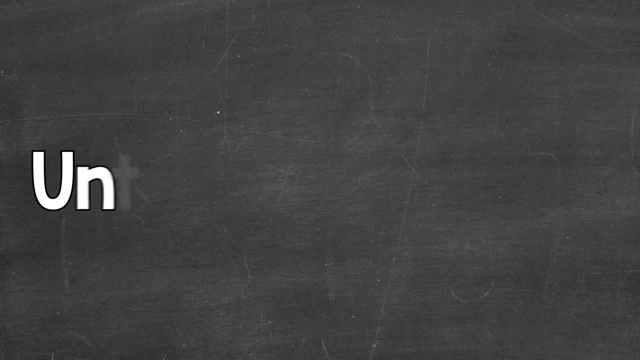 I drop the link to the six through ten perfect cubes and cube roots video down in the description, along with some other related videos. I hope that helped. Thanks so much for watching. Until next time, peace. 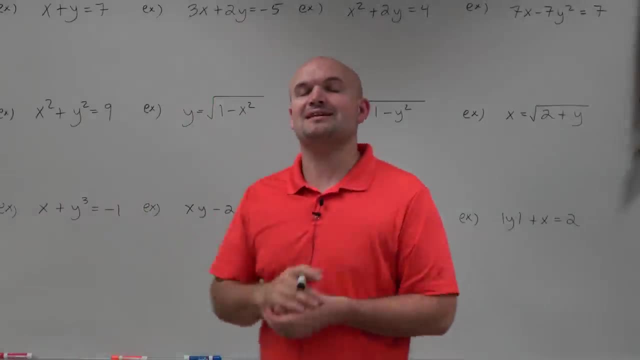 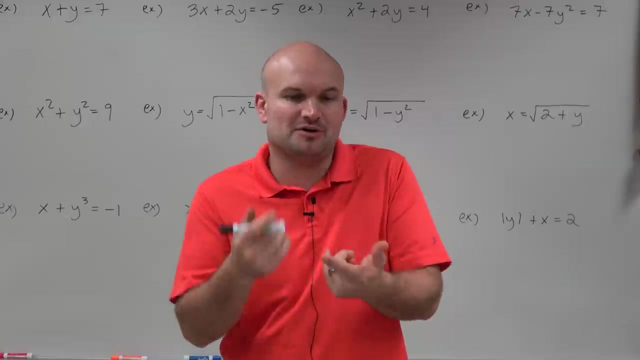 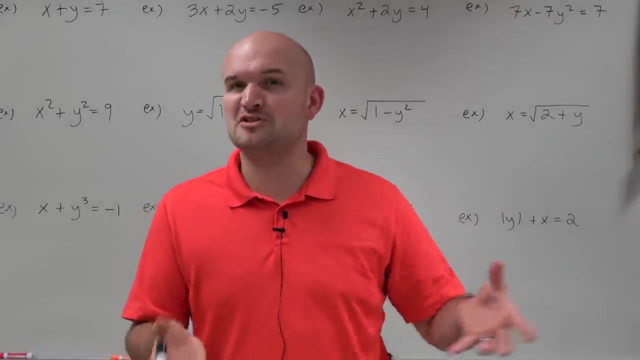 Welcome, ladies and gentlemen. So what I'd like to do is show you how to determine if an equation is a function. So previously we've looked at tables, graphs, mapping coordinate points to determine if they represented a function, And it was relatively simple to. 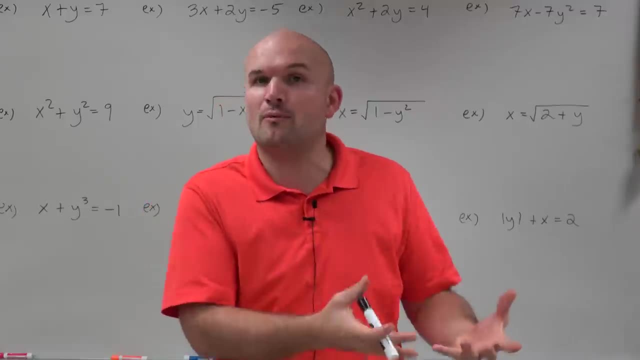 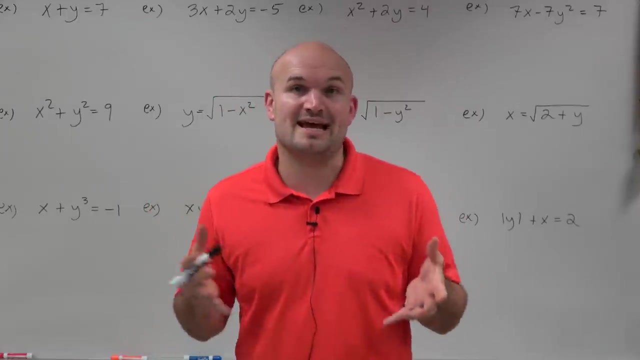 identify that Every x had to uniquely map to one y, Or we could apply the vertical line test, And it was rather simple to be able to determine if a relation was a function or not. So now what we're going to be doing is looking at equations And basically what? 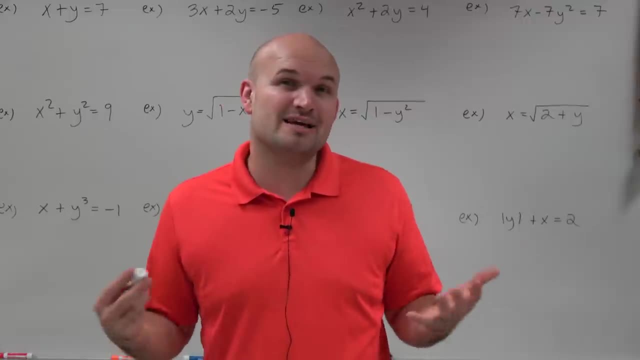 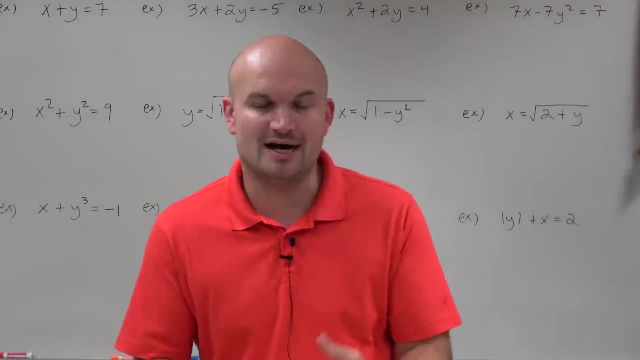 we're going to try to do is solve for y uniquely. And as long as y can be solved uniquely, then we know that for every x value that we enter into the equation, or at least every independent value, that our y value is going to be unique And we'll come across, we'll kind of talk. 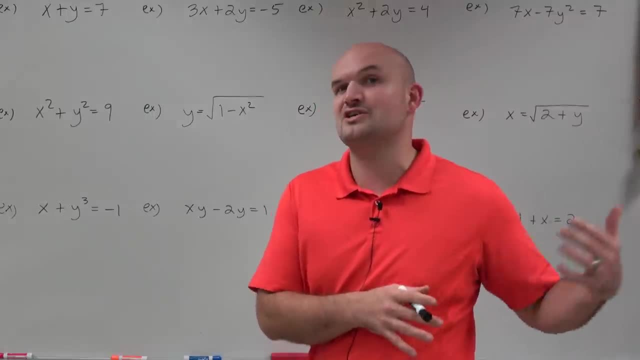 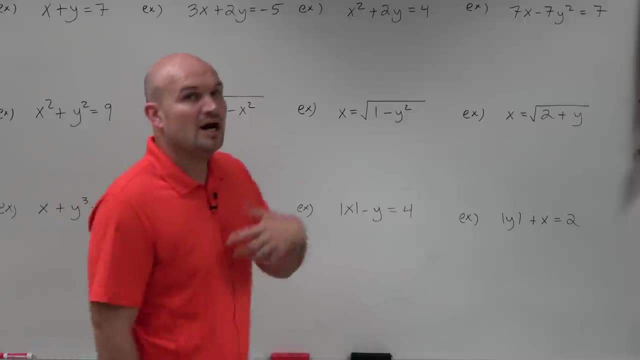 about some problems where we start seeing when the equation starts to not be a function. But the first step we really want to do for all of these problems- we're going to basically be going through the same process- And that is to isolate the y and make sure that it. 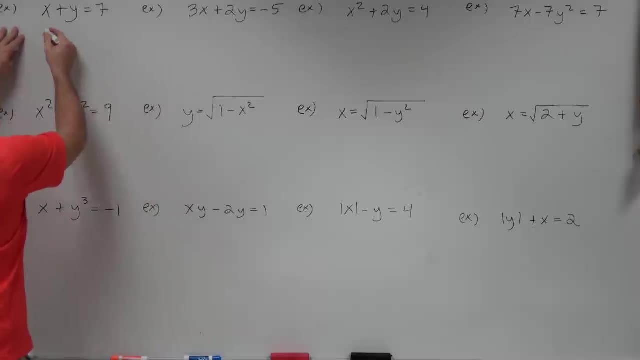 can be solved uniquely. So in this example here I can just solve: subtract an x here and I get y equals. you can just write the negative x in front, negative x plus 7. And therefore that is. I have solved for y uniquely For every x value, it doesn't matter whatever. 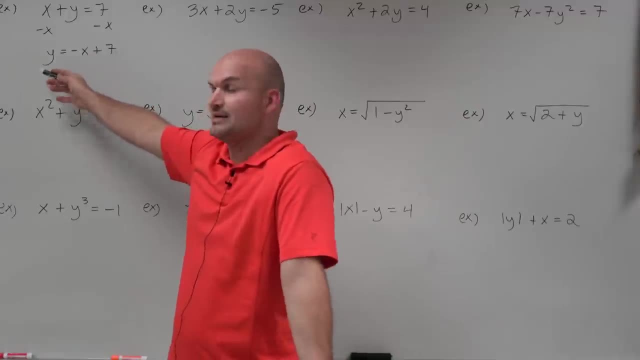 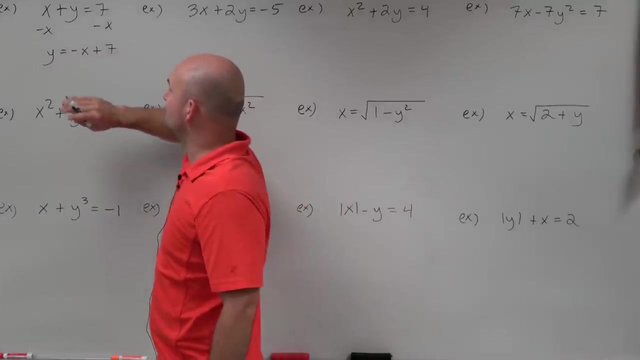 number. I plug in for x. right, that's my independent variable. y is my dependent. For any value, I plug in for x. I'm always going to get one unique answer for y. So therefore, that is a. I solved for y uniquely, So we'll call that a function And I'll just